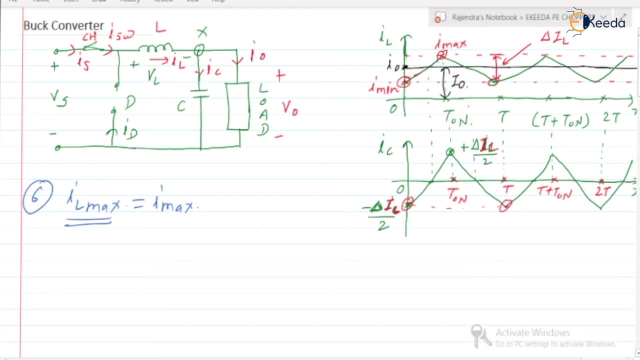 expression for I max in terms of I max, in terms of, yes, the load current, that is, the capital I 0 or the capital I okay, capital I 0 or capital I okay. and can we write the expression for this current capital I or capital I 0? you can say okay and this repellent inductor current. 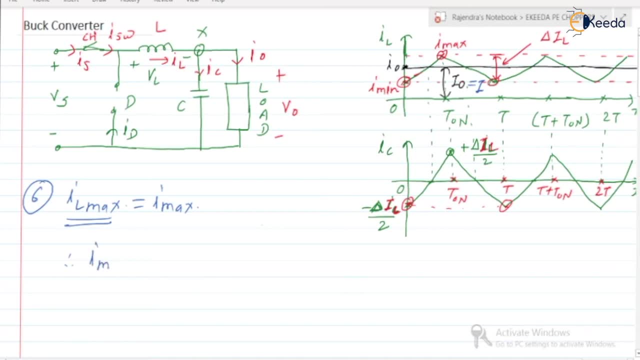 yes, we can write I max. therefore, we can write: I max is equal to what, I L max is equal to what. yes, we can write it as a I plus delta I L or delta capital. I L right, delta I L by 2. right is the I plus delta I L by 2. are you getting the point? 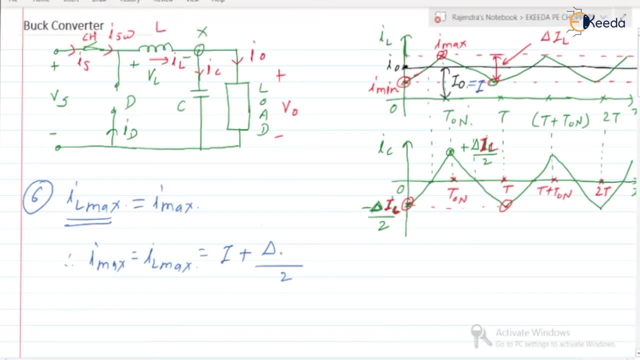 right. delta I L by 2. are you getting the point in check once it is the I plus the delta I L by two. delta L means what the difference between these two? so these indicate delta L, this indicates delta L. okay. so fifty percent of this means what? only this much length. okay, so it is I. 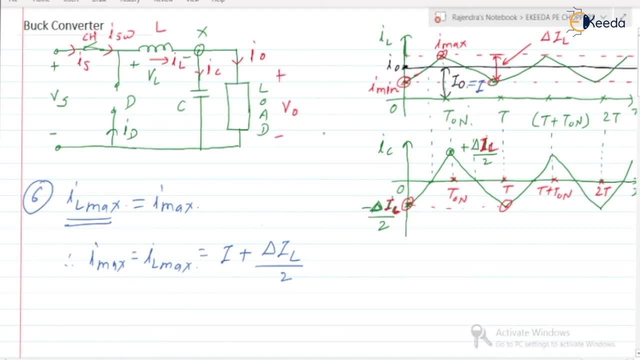 plus I is nothing but this magnitude, I plus delta, I L by 2 is nothing but I max. okay. similarly, for the seventh, can we write it as I min or I L min. minimum value of inductor current. okay, inductor current minimum value is nothing but I. 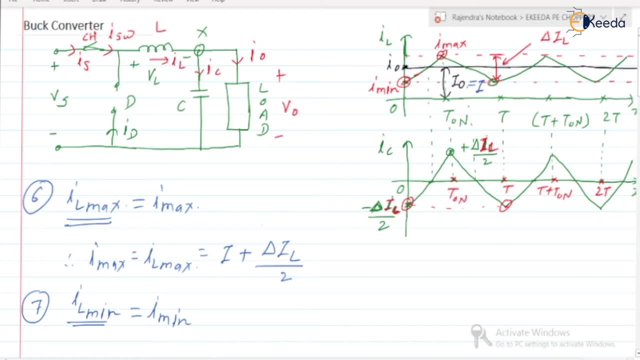 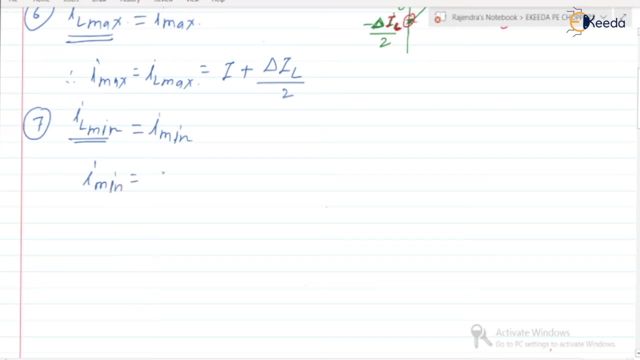 min is nothing, but i mean right. so here we can write: i mean is equal to yes, similar to that of imax. yes, it is a. i mean is equal to what il mean. il mean is equal to what i minus delta il by 2. can we write in this way? yes, if you check, i is nothing but this current, okay, minus delta il by 2. 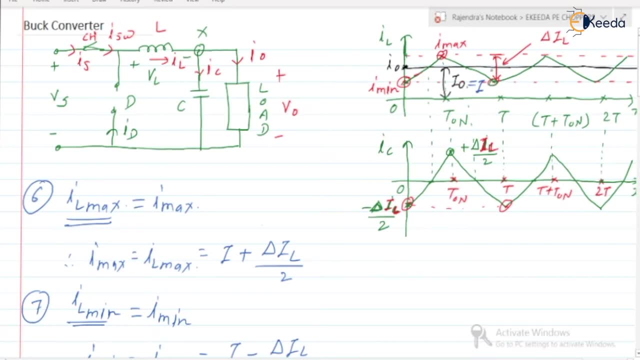 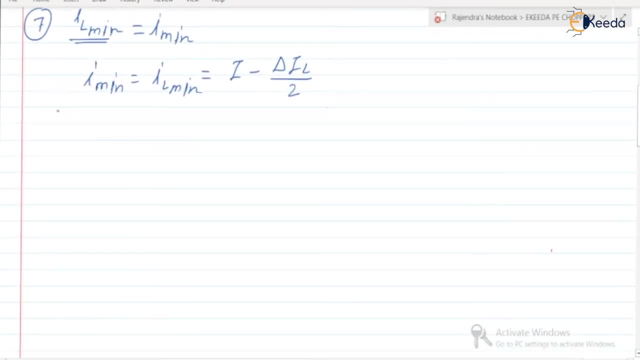 delta. il means this value, 0.2 means this term. okay, so i minus this value, i minus this length: 50 percent is nothing, but i mean is nothing, but i mean, is this clear? next, the eighth parameter we are having is: yes, source current, right. source current is okay. source current: source current. 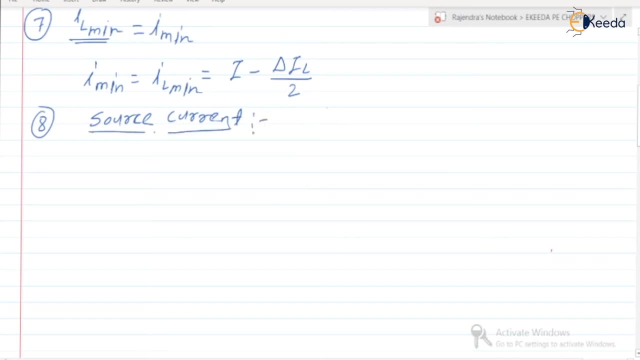 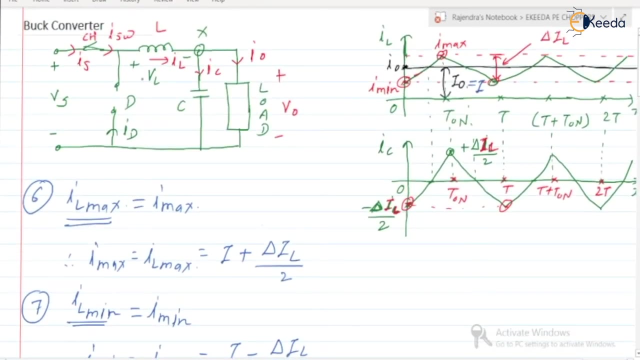 right. so here, if you check the circuit, yes, we are having the supply and we are having the load, okay, next, what is the power consumed by the inductor and capacitor? real power? it is a zero diode is ideal element, which is also the ideal switch. okay, so, whatever the power supplied by the source is nothing but the power. 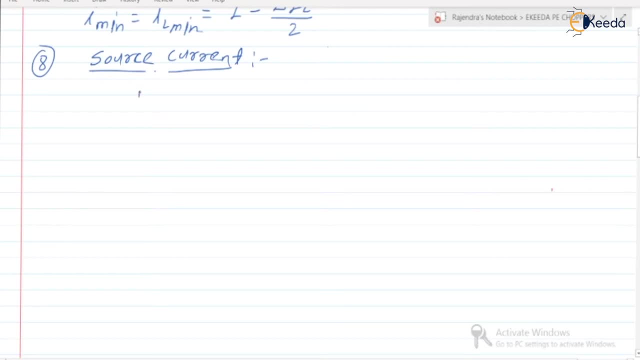 consumed by the load. yes, so can we write it as: p in is equal to p out, right? input power is equal to output power, right? is this clear? so for finding the source current, when it equals the input current, it is theassy degree to, etc. okay, what is the input power? it is the vs into. 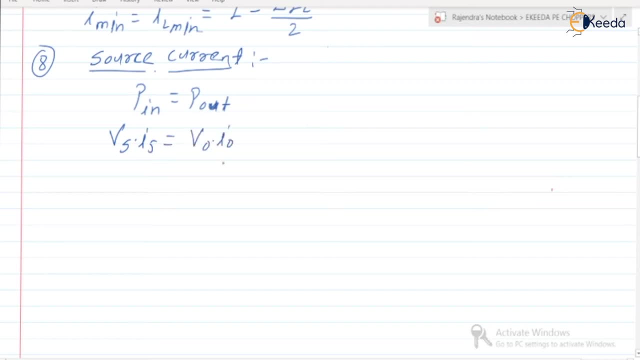 is okay, is equal to what v0 into i0, right v0 into i0. so therefore we can write: is i s is equal to what v0 into i0 divided by vs. okay, but what is the v0? v0? is d into vs? we already derivative to i 0 divided by vs. okay, so vsvs will get cancelled, so it's equal. 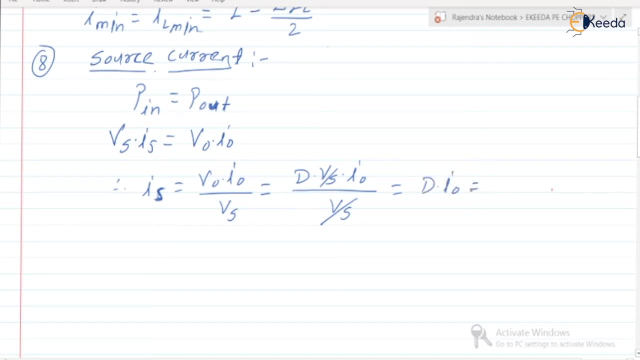 d into I0.. But what is the load current I0? It is a constant current, So it is a d into I0 or we can write it as a d into I. also. Is this clear? Load current is the constant current, So. 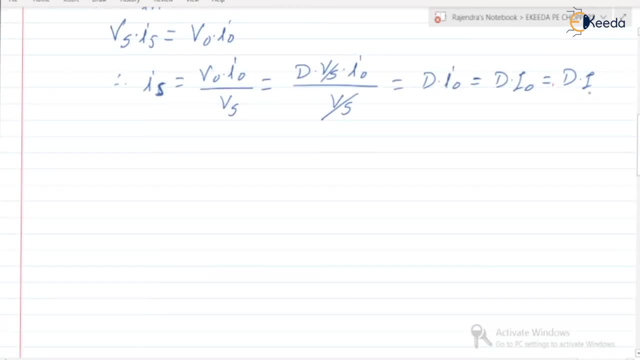 now, if the load current is constant current, so duty cycle into the constant current. that is nothing but your Is. So this is giving. because this, what is the average value of Is is equal to duty cycle into load current average value. What is the load current average value? Load current. 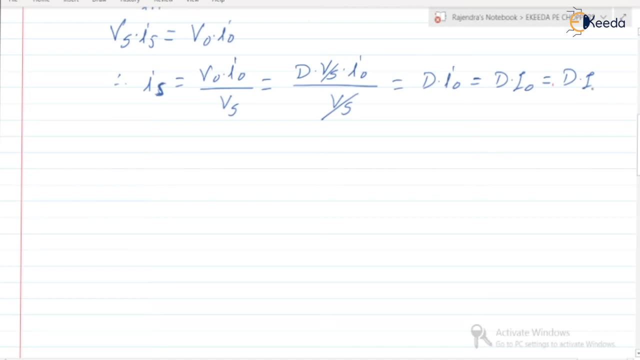 average value is load currents magnitude only because load current is constant current here, okay, So here, indirectly, this is given: giving Is average, V right, we are getting Is average okay, So therefore we can write: Is average is equal to what D into I0 average, okay, So 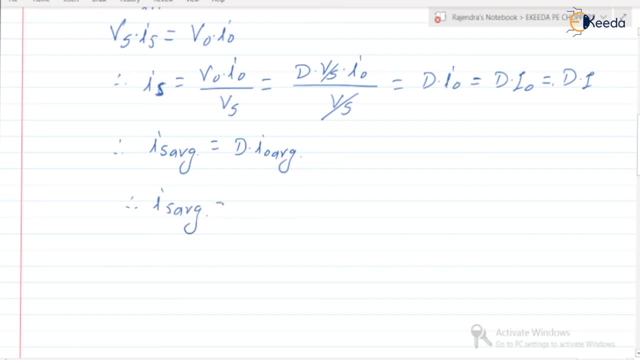 therefore, Is: average is equal to D into I or D into I0.. Is this clear? Okay, So this is about the source current. This is about the source current. okay, Next, switch current average and RMS value. okay, Next. now is point number 9,. switch current. okay, Switch current. 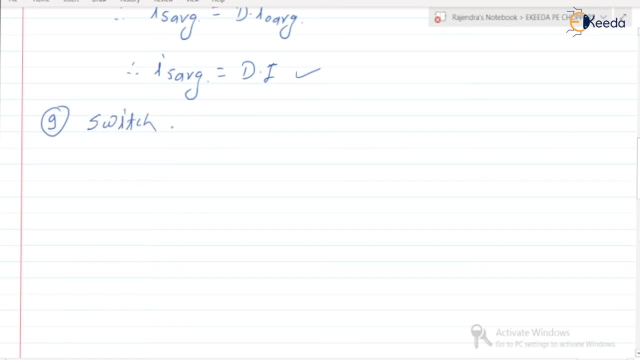 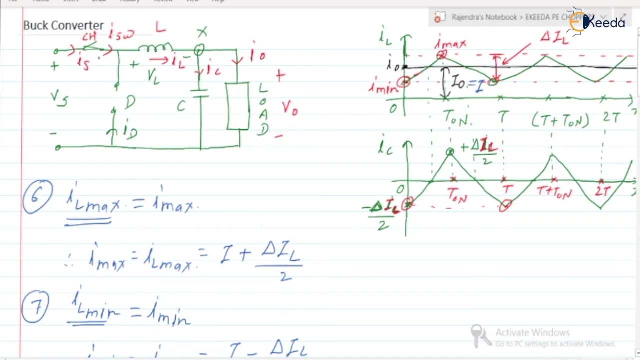 switch current, okay, average and RMS. average and RMS okay. So here, switch current means what Is W, okay. So can you find the Is W average value When switch is in the on state. when switch is in the on state, if you check, yes, switch is in the. 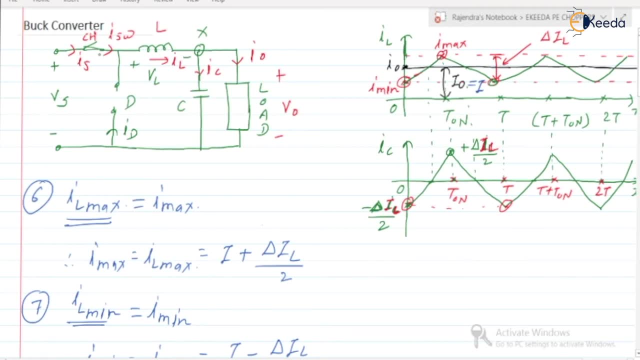 on state at that time. yes, whatever the IL we are having, the same Is W will be there, okay. Next, when switch is in the off state, Is W will be 0, okay. So here can we draw the waveform for. 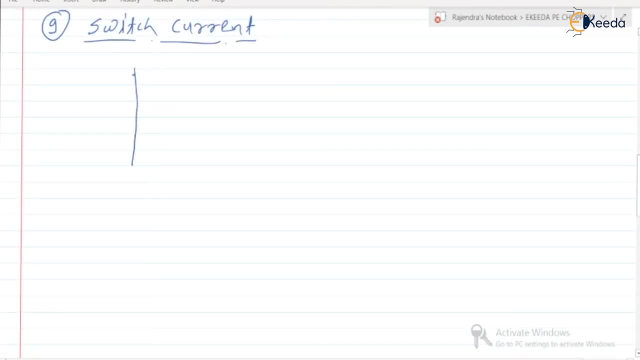 the Is W: Yes, we can write, we can draw the waveform for the Is W. it is Is W. yes, during 0 to T1, this same as that of the IL, so time T0,. yes, I mean to I max. it is increasing till this T1, okay Again, after that it will be 0,. 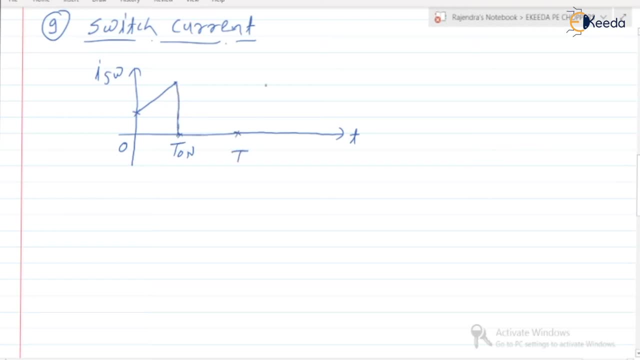 after that it will be reaching 0, T1 to T. okay, Again at T, it is again at capital T, it is again I mean to I max, it increases and till T plus T1, right, this is value we are having. 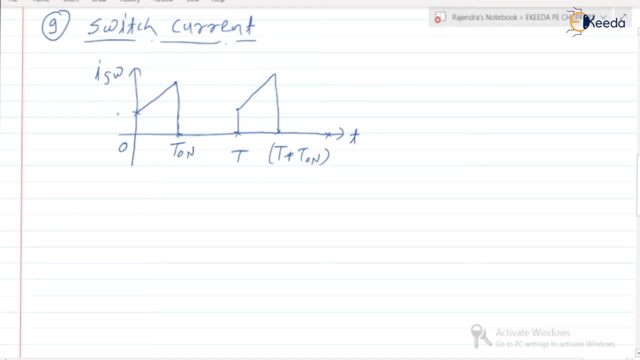 and at 2T it will be again till 2T. it is 0.. Okay, So this value is nothing. but I mean this value is nothing, but I max, okay. So here the switch current is non-zero, only from 0 to T1, from T1 to T. the switch is open, so switch. 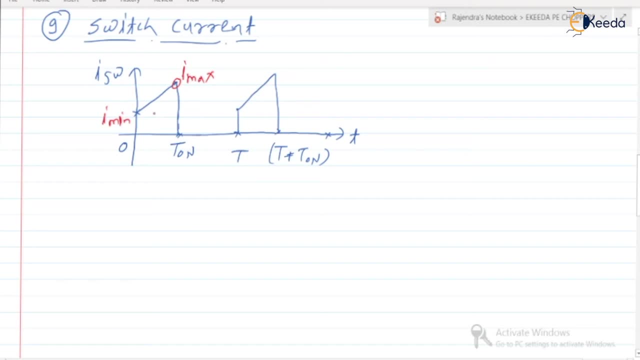 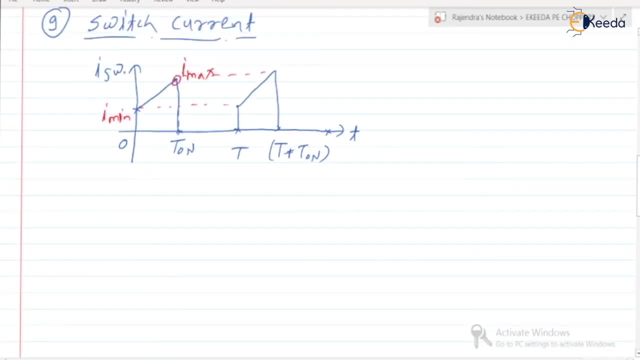 current is 0, right Again from T to T plus T1, it is again changing from I mean to I max, I mean to I max. is this clear, okay? So now further, can we approximate this waveform? 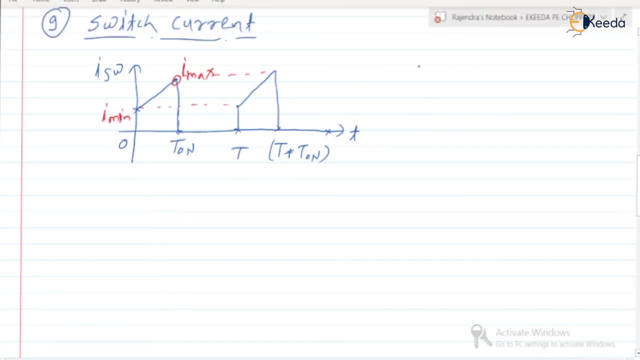 as can we redraw this waveform as I am drawing here? Yes, further, we can redraw this network, sorry waveform, as this is a switch. current waveform time: T: 0,. okay, Okay, So it is like average of these two right, average of these two is nothing but this value. 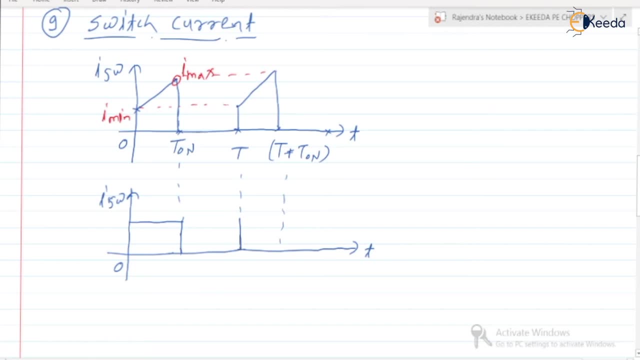 and here it is a 0 value. right Further it is the average of these two, and again, okay, average of these two. okay, So it is like a I mean plus I max by 2,. okay, till T1, here. 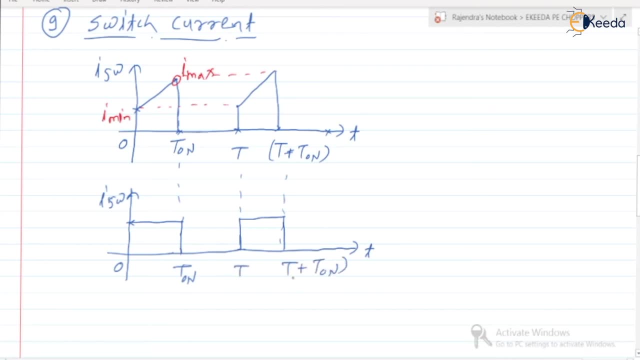 it is T and here it is T plus T1, are you getting the point? okay, So 0 to T1, it is the average of I mean and I max, average of I mean and I max, all right, So what is the? 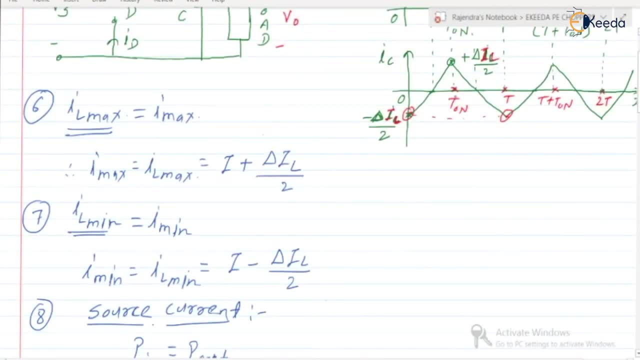 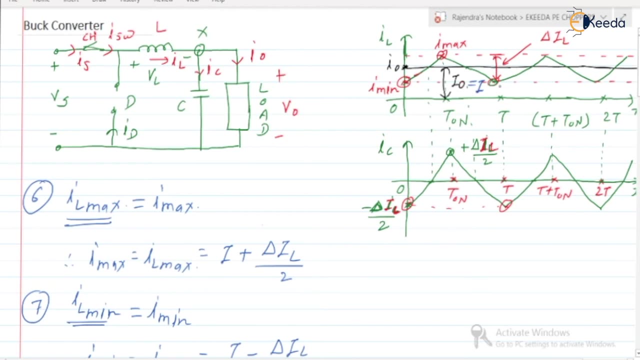 average of I mean and I max. if you check the average of I mean and I max right. So waveform, what is the average of I mean and I max right for this shape? what is the average? it is I0, capital I: okay, So we can say that it is a load current right which is equal to: 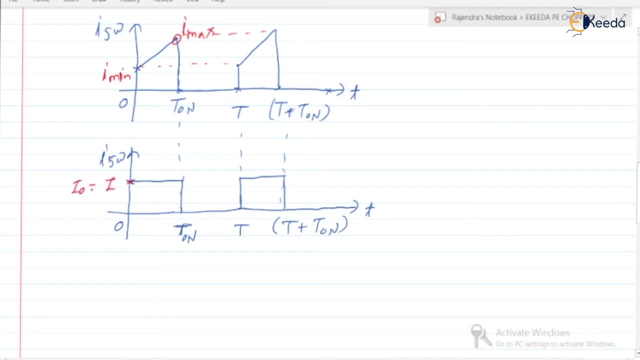 capital I, which is equal to I0,, which is equal to I0,. are you getting the point right? because this is nothing but the average of these two right average of, I mean to I max. okay, So now, if this is the case, then can we find the value of ISW average? yes, I am writing here. 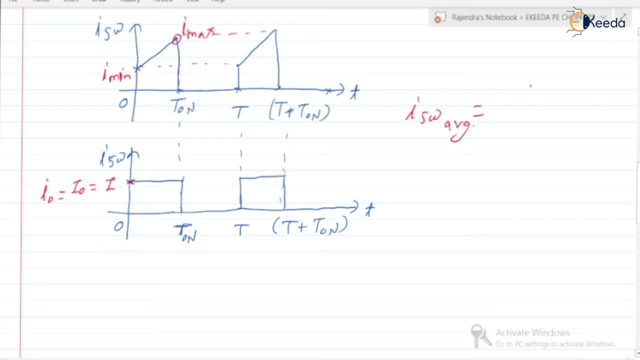 average is equal to what. yes, average value of the switch current is equal to what. it is a. 1 by T. integration from 0 to T1,. what is during 0 to T1, what is the current? it is a I into DT. 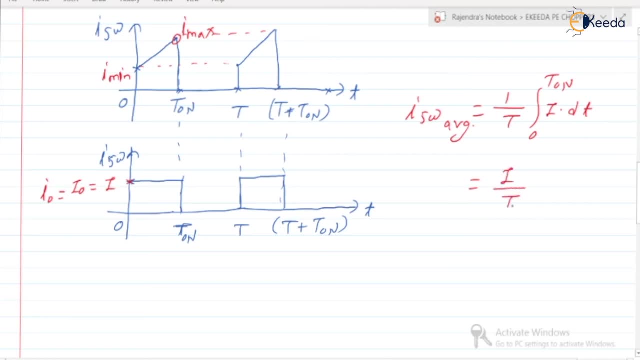 okay, So is equal to what. we can write it as a I upon T into T1, so it is a T1 by T, that is, a D into I. this is what ISW average right. So what is the average value of the switch current right, which is same as that of the? 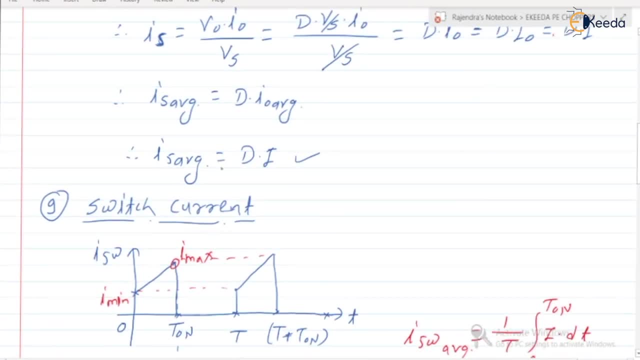 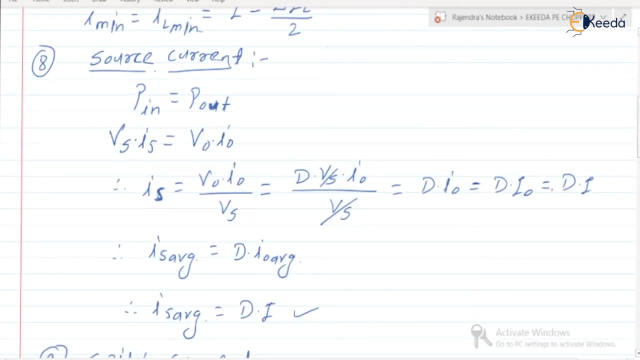 average value of the source, current yes or no? right, it is same. IS average is same D into I. ISW average is also same. that is a D into I. because if you check the circuit, if you check the circuit, you will understand when switch is in the on state. at that time IS and ISW both. 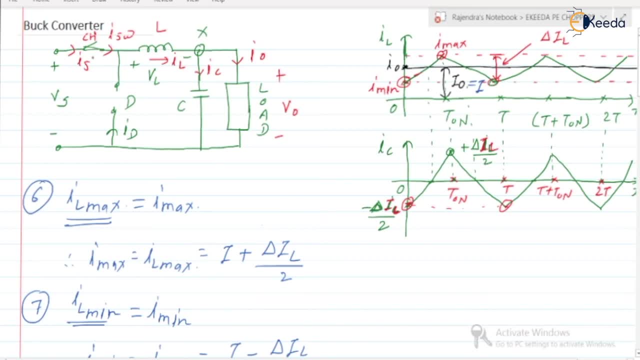 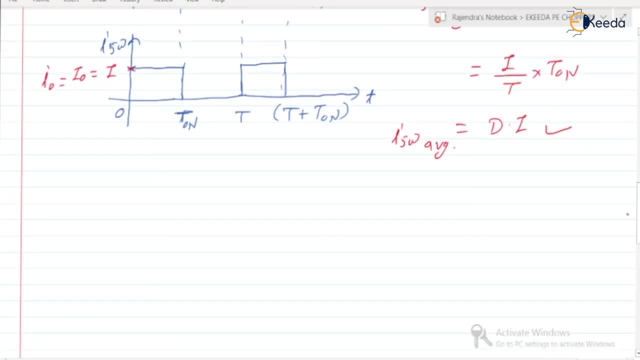 will be non-zero, right, and both will be same. and when switch is in the off state, ISW and IS both will be zero. okay, So ISW and IS both will be having the same waveform. okay, So ISW average. 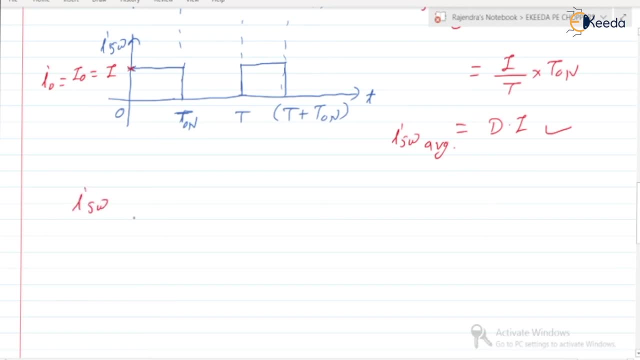 is same as DT into I. next, can we find ISW? that is a switch. current RMS value: yes, it is equal to 1 by T integration from zero to T on: yes, during zero to T on, it is a. 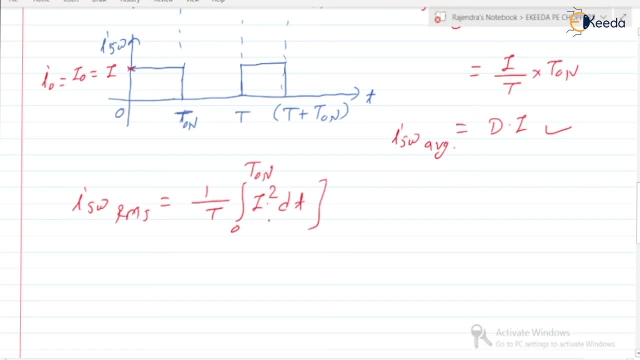 I square into DT to the power 1 by 2, square root of mean of squared value. so is equal to what we can write I upon root T into under root T on. is this clear, okay? So under root T on by root T is nothing but root T into current. I right, this is nothing. 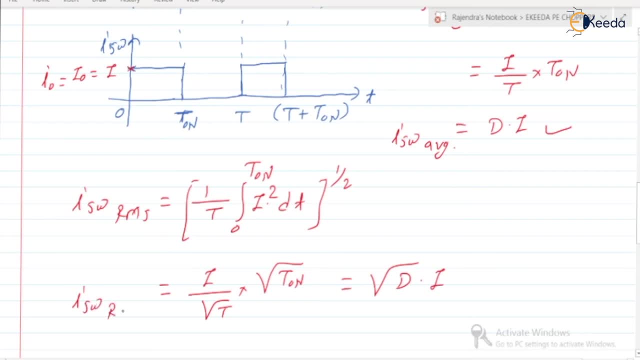 but the ISW RMS. RMS value of the switch current. RMS value of switch current. is this clear? it is a root D that is a duty cycle into I, duty cycle into I. okay, So this is nothing but the RMS value of the switch current, next diode, current average and RMS value. 10 number. 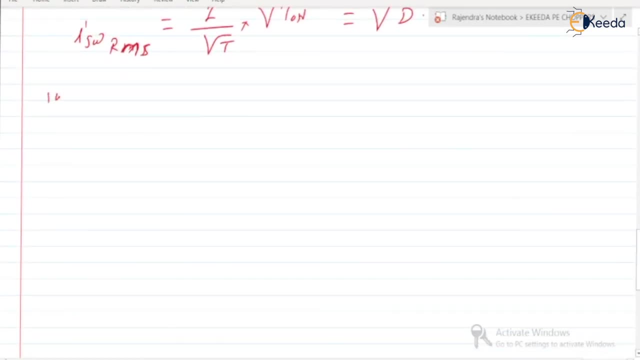 okay, we can find point number 10.. Diode current: diode current average and RMS. right diode current average and RMS. So if you change the circuit operation during zero to T on what is the diode current? this 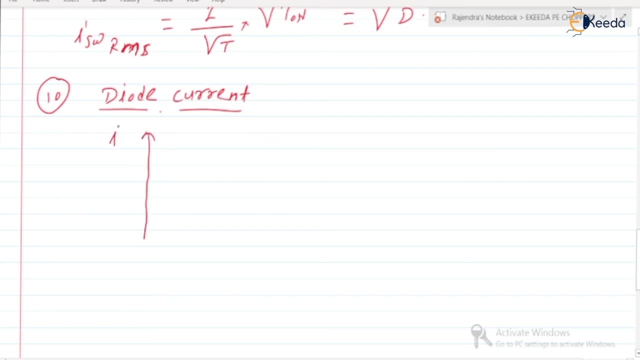 is zero, right, so we can draw the waveform for the IID: diode current, IID right. yes, T, zero. okay, If you check, diode current is zero right. diode current is zero because during zero. 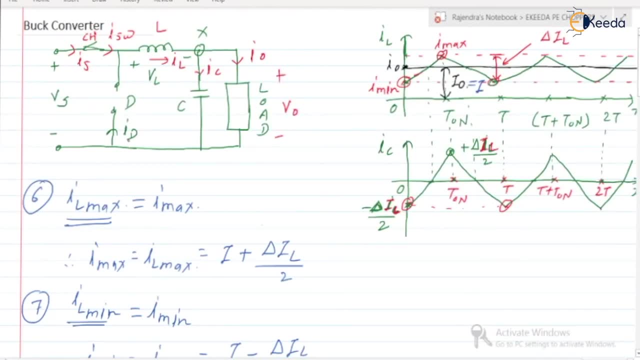 to T on. yes, our switch is in the on state diode is in the reverse bias mode, so IID will be zero, okay. During T on to capital T. during T on to capital T. if you check, switch is open, okay during. 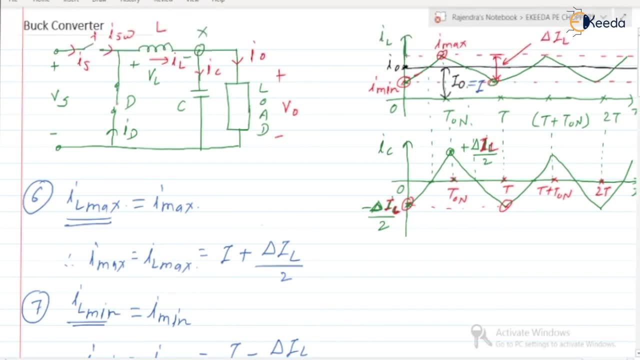 T on to capital T. the switch is open. diode is in the on state. at that time can we write: IL is equal to IID. yes, IL is equal to IID. okay, So IL is IID. means what IL, whatever the waveform we are having. 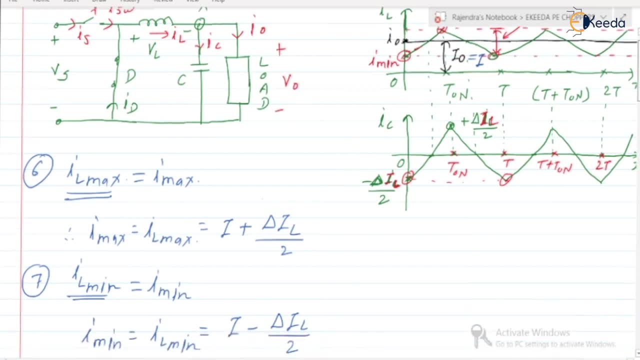 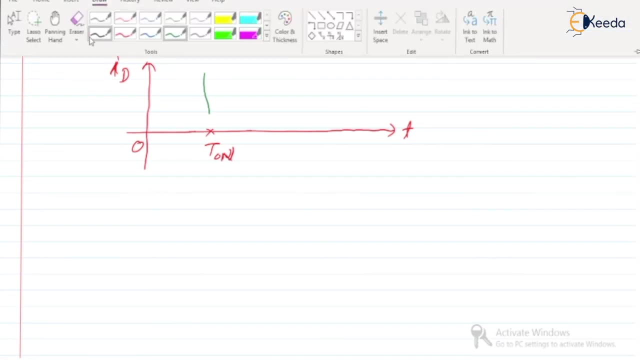 The same will appear for the diode current. okay, that is IMAX to IMIN. okay, so here, diode current waveform, it will be like IMAX to IMIN. it is changing from IMAX till IMIN. okay, to diode current waveform. it is changing from IMAX till IMIN. okay, here it is capital. 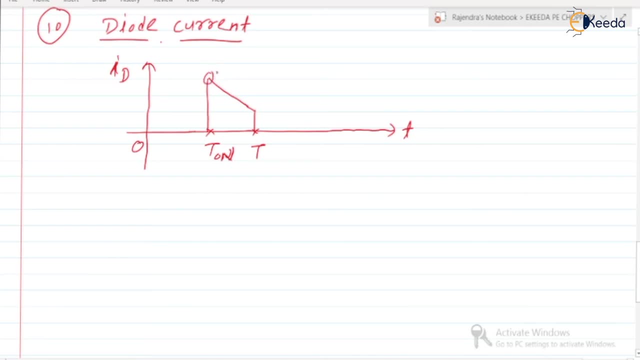 T, okay. so this is IMAX. One is IMAX. One is IMAX. One is IMAX. Okay, and again, from T to T plus T1, it is a zero, and after that again it is a non-zero. 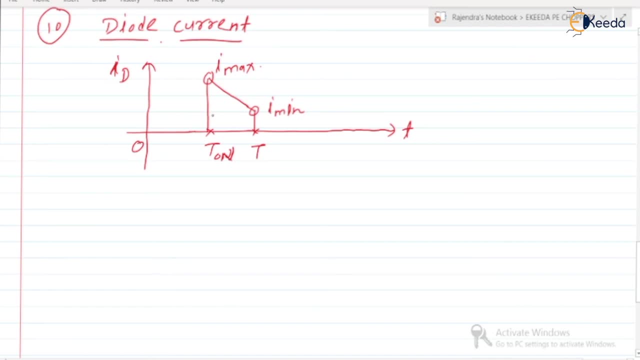 okay, same same cycle repeats, okay. so for this can we further redraw this waveform, as what is the average of this IMAX to IMIN? it is I0, only right, or the capital, I, only right. we can redraw this as time T: 0.. 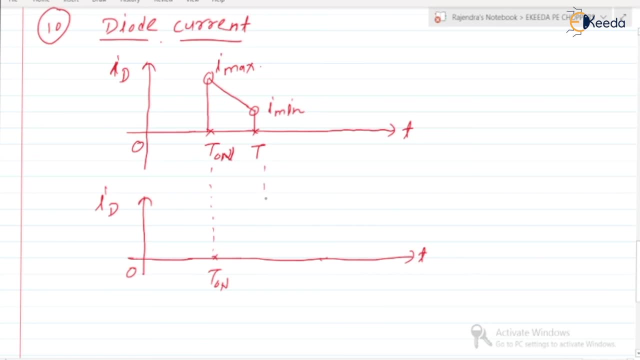 This is t1,, this is capital T, and here, where is the average value? What is this average value? Average value is: yes, this average value is nothing but S capital I, which is equal to I0. only Now, for this case, for this waveform, can we find the ID average value of the diode current. Yes, is equal to what? Average value of diode current is equal to 1 by T integration from t1 to T. 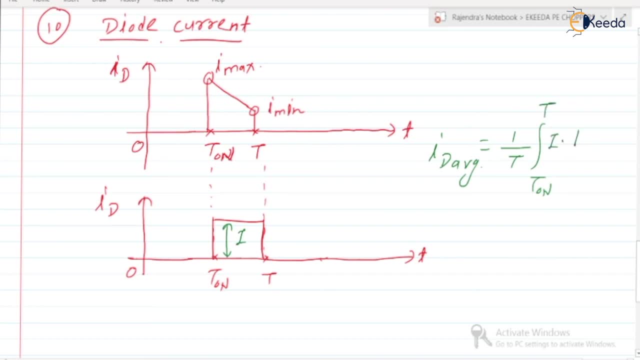 T1 to T. yes, it is capital I into dt, So this can be written as I by T into T minus t1.. Okay, so further. this can be written as I upon T into yes. T minus t1 means what D into T. 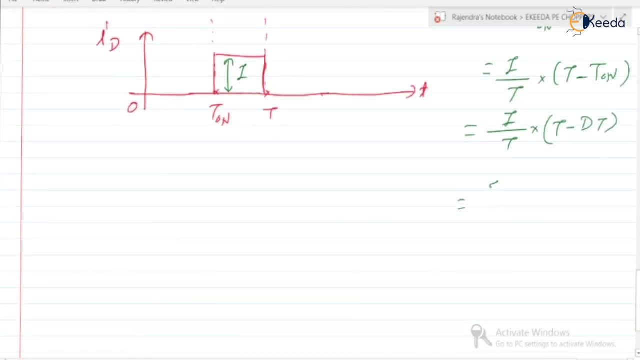 Okay, so we can take T common. So it is like I upon T into 1 minus D into T. T. T will get cancelled, So it is equal to 1 minus D into I. That is nothing. but what ID? average Average value of diode current. 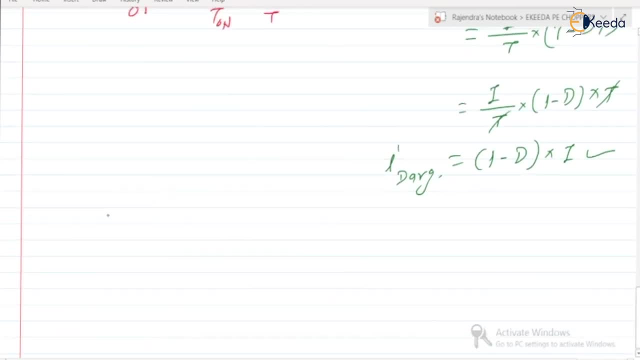 Okay, Is equal to 1 minus D into I, right? Similarly, can we write ID RMS- Yes, I am writing here ID RMS. ID RMS: square root of mean of squared value. So this is 1 by T integration from t1 to T, right.